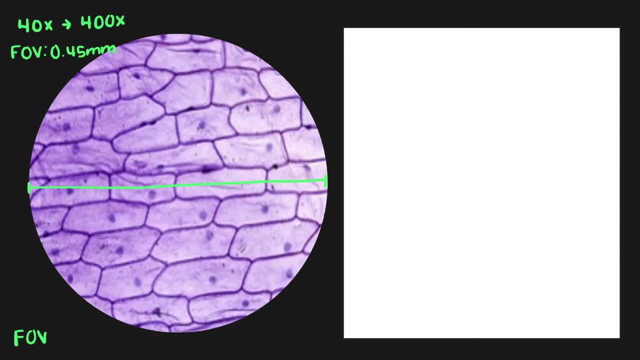 which we do. we can do that down here. our field of view is 450 micrometers, all right, so we're just going to erase this. so now we're going to pick a cell to draw, and i'm going to pick this one in the middle. it's a good little shape. it's in the middle, so it'll. 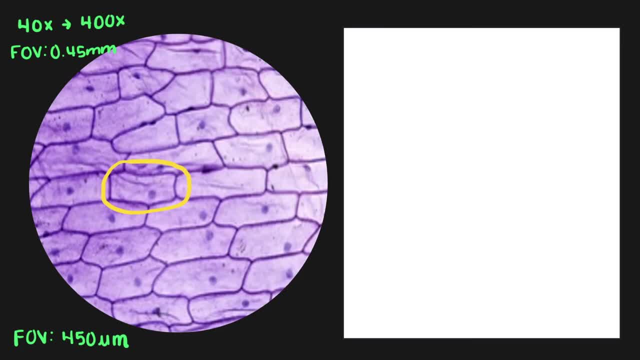 be easy to estimate our fit number which we'll get to next. so we want to draw our biological drawing to take up most of our page, at least half, if not two-thirds. and when we do our biological drawing we don't want to do any shading, we want to try to do all connected lines. 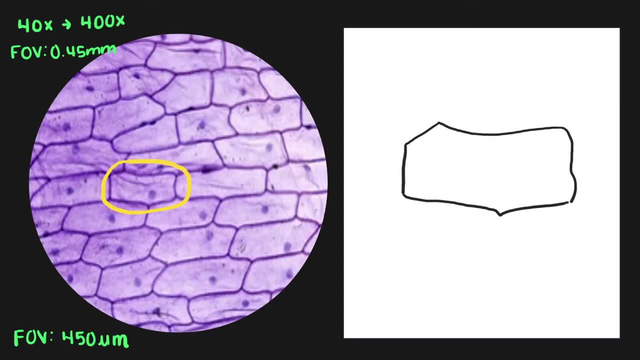 so we'll just do the right way and we'll just do 10-10 and we'll just do one more. and we have a little nucleus here, and to show that that is darker than the rest of the cell, we're just going to do some stippling in there. so we're not going to worry about labeling at all. 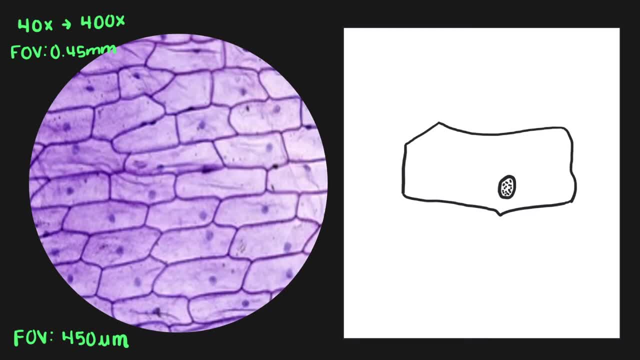 we're just going to have our bare bones drawing here. what we want to do now is estimate the fit number, and that's going to be how many times the cell that we've drawn will fit across our field of view in its longest dimension. so we're going to do a little stippling in there and we want to do our. 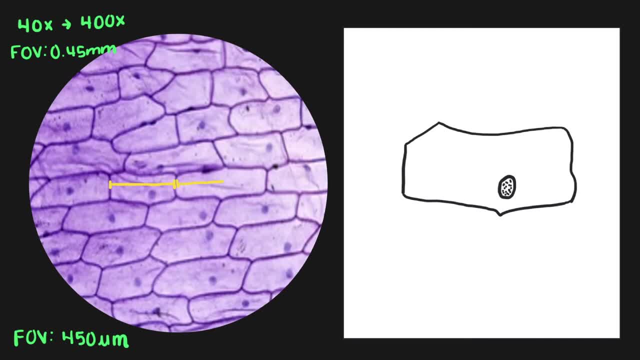 So if we were to stack this cell end to end, how many times would it fit? And you can and you would ideally measure this, but we don't have a ruler on this app, so we're going to just estimate. So it looks like here we have one, two, three, four complete cells, probably five with the 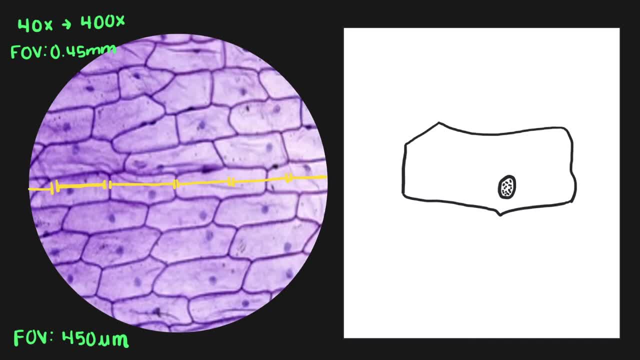 end bits there. So we're going to say for this drawing that our or for this cell that we've picked, that our fit number is five. Our cell will fit across that field of view five times. And now we're going to look at why that matters in terms of calculating the size of our cell. 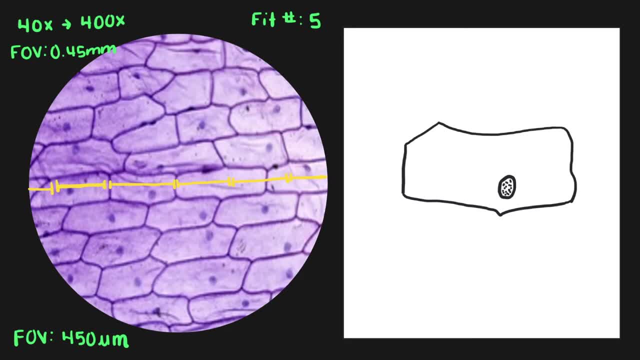 as well as why that matters in terms of calculating the size of our drawing. So we're going to start with cell size. So we want to know how big that cell actually is, And we don't need our drawing for that, because all we really care about is our field of view. 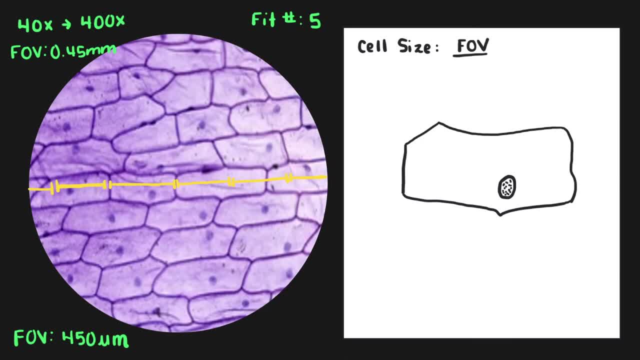 over our fit number. So our field of view is 450 micrometers And our fit number is five. So when we do that in our calculator, 450 divided by five, we get a cell size Of 90 micrometers. 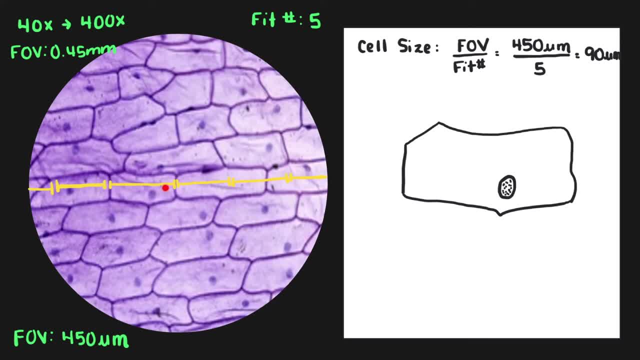 So that means that this cell in this dimension is 90 micrometers long. So now that we know that, we're going to be able to figure out how big our drawing is compared to the actual size of the cell in reality, not the size of the cell in this. 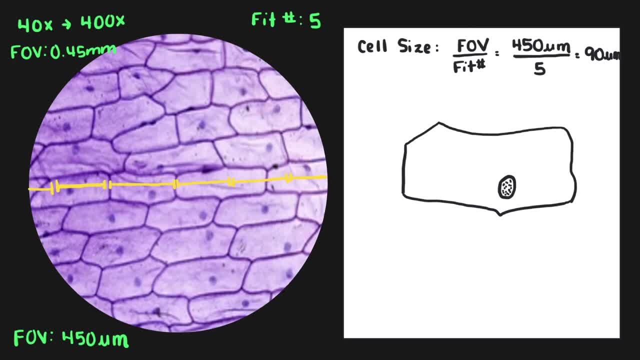 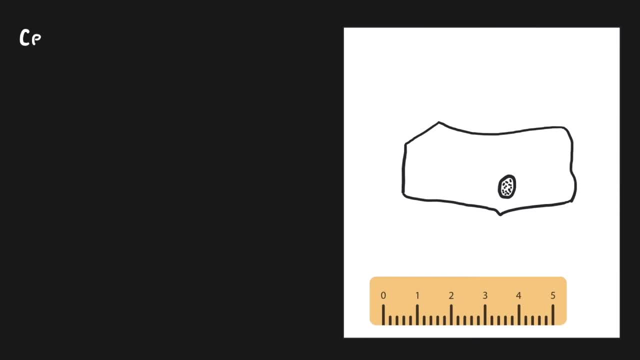 microscope image, but the size of the cell as it exists in the onion itself. Okay, So we know that our uh cell size is 90 micrometers, And now we want to see how big did we make our drawing here compared to the actual size of the cell? 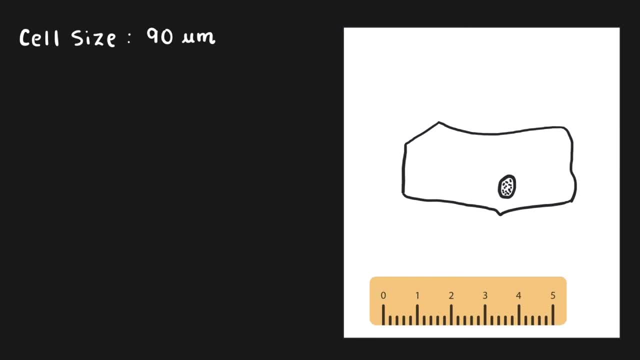 And for this we need a ruler, because we're going to actually measure our drawing. So we're going to take our ruler and we're going to place it over our cell in the same dimension as what we measured- the fit number- And we see that our drawing 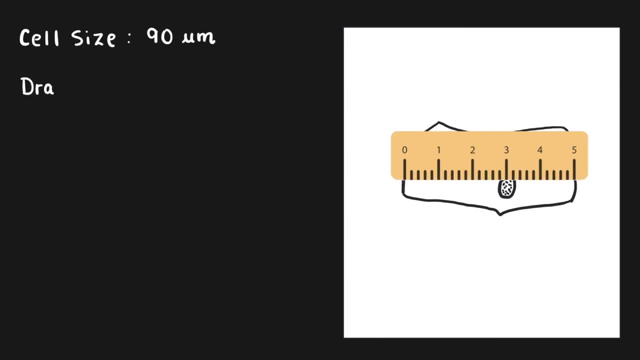 is exactly five centimeters. Now we see these are different units, So we obviously want to convert five centimeters into micrometers. We can do some unit conversion for that. So five centimeters And in one centimeter there are 10,000 micrometers. 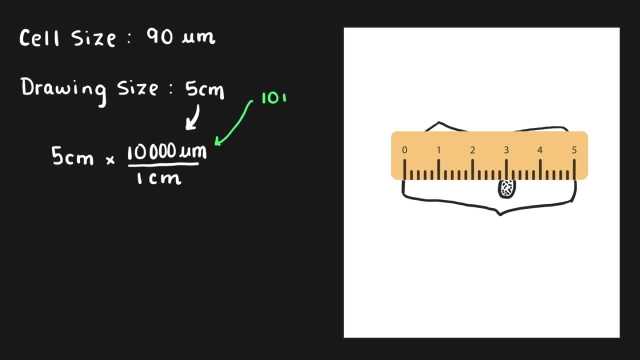 And we know this number because there are 10 millimeters per centimeter and 1,000 micrometers per millimeter. So we multiply those two conversion factors together, we get to 10,000 and we see that our centimeters here are going to cancel. 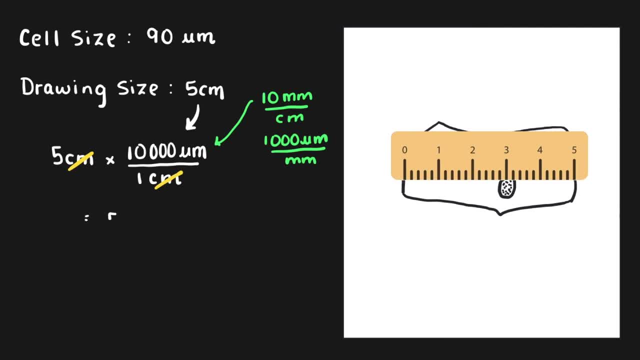 So we have five times 10,000.. So we have five times 10,000.. That equals, or, sorry, yeah, five times 10,000.. That equals 50,000 micrometers. That's how big our drawing is. 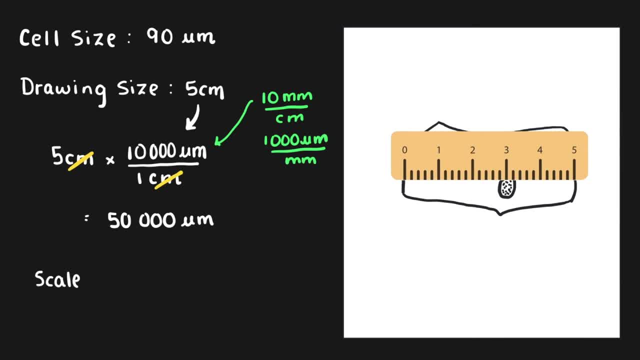 So now you can do the scale of our drawing. That's going to be 50,000 micrometers. How big our drawing is- over 90 micrometers. how big the cell is, And we find that we've made our drawing 556 times bigger. 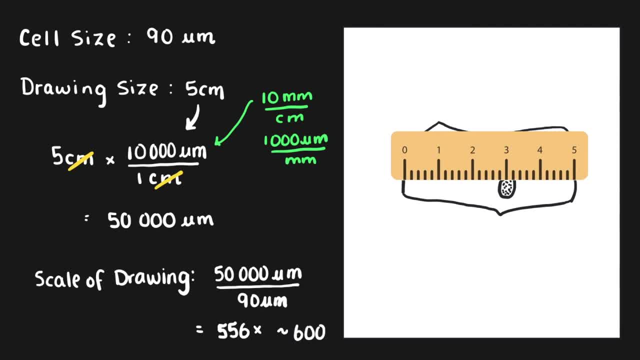 and we're going to round that up to 600 times bigger. So our drawing is 600 times bigger than the actual cell. Now we want to make a scale bar here. So along our ruler we're going to draw ourselves a one centimeter line. 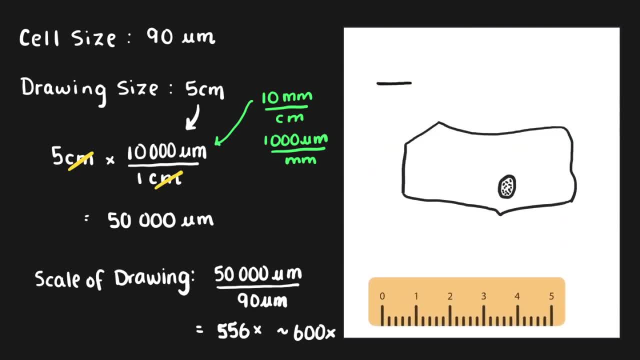 Let's move the ruler out of the way there. So our scale bar is going to be smaller than our drawing And we want to figure out how big or what, what number, to put above our scale bar here to indicate to anyone looking at the. 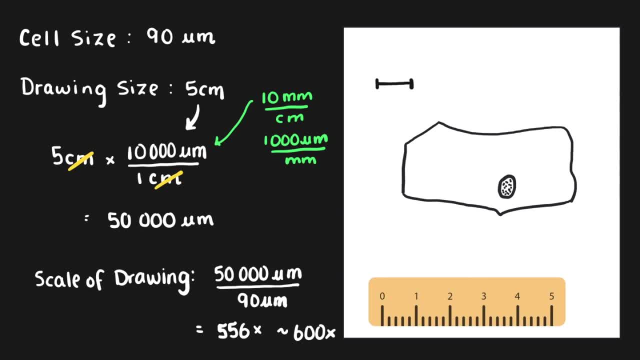 drawing, how big that drawing or how big that cell is. So what we're going to do is we're going to say: our scale bar is one centimeter and our drawing is five centimeters in total, And we're going to just put X for micrometers. 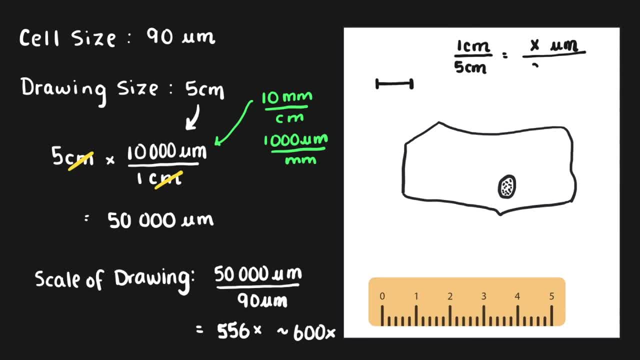 So how many micrometers does our scale bar represent when our cell in total is 90 micrometers? So here we have our scale bar length. Here we have our drawing size. This is going to be the number we put above the scale bar. 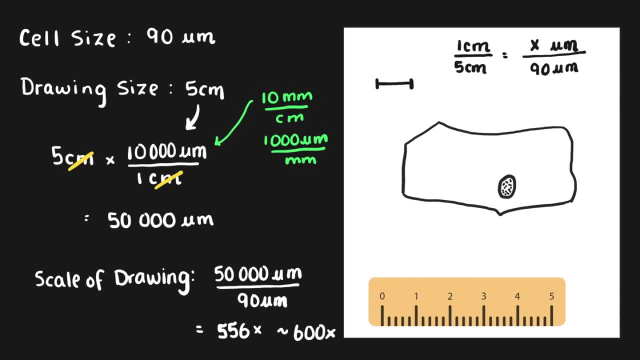 and this is the actual cell size And so we can rearrange. X is going to equal one times 90. And so we're going to say our scale bar is 90 over five And our units are going to be micrometers, because our centimeters here will cancel. 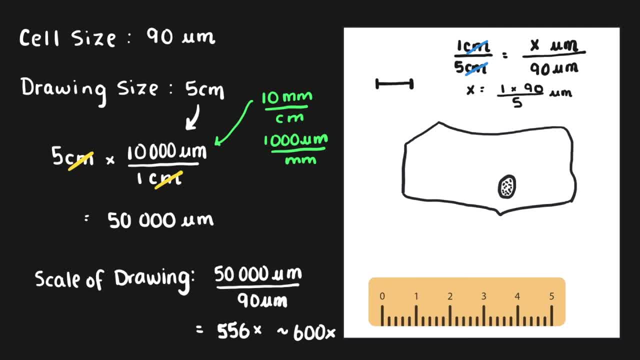 And so 90 divided by five is 18.. So this scale bar represents 18 micrometers, And so if we were looking at this drawing done, we could measure our scale bar. So we can see that our scale bar is 18 micrometers.